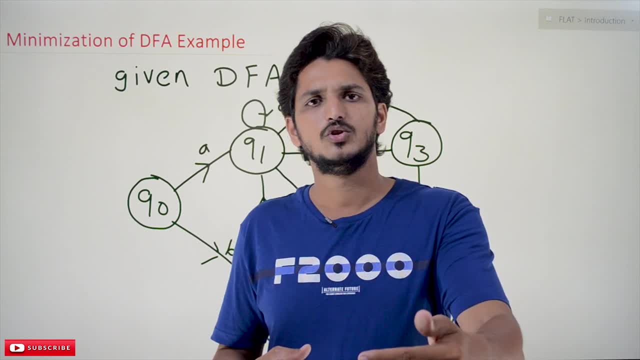 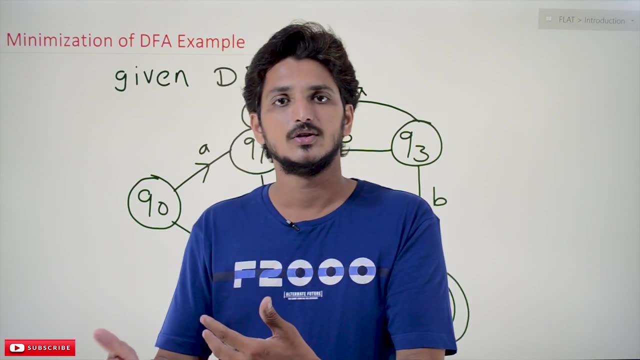 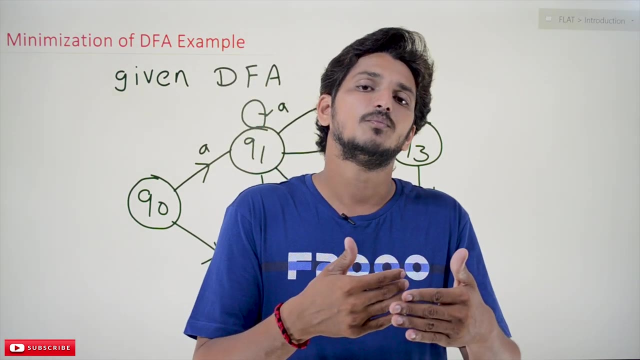 a DFA, You can define your logic on your own. You may write your logic in a lengthy manner. Maybe some other person will write a logic in a short way. So you may not get whenever you convert your NFA to DFA you may not get the shortest possible logic. That's why, if you take 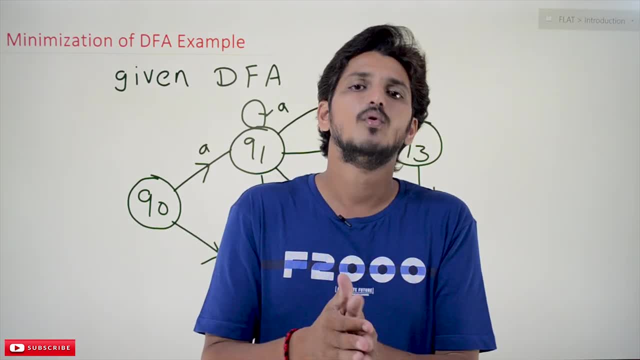 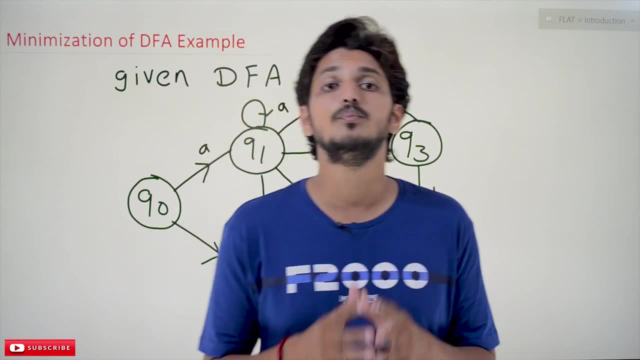 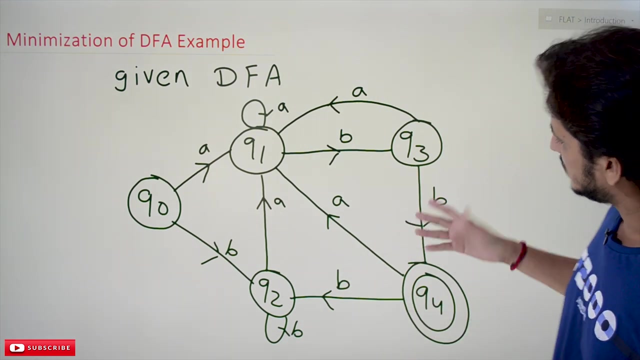 any DFA if you, after minimizing it, we'll get the shortest logic possible. So for that we need minimization. Let's try to understand how to minimize our DFA. Coming to the example: given this DFA, some DFA has been given It will accept. I guess this will accept the strings that 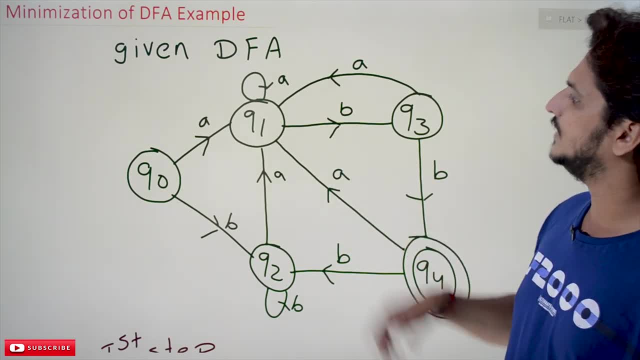 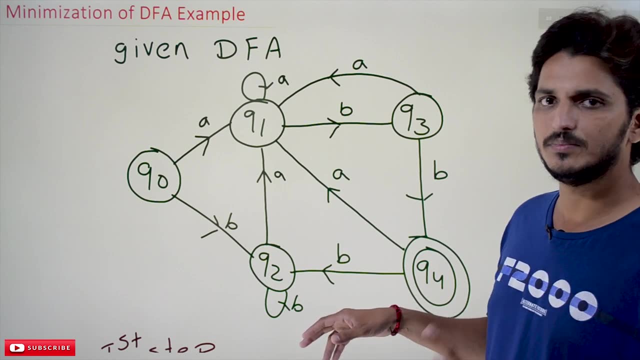 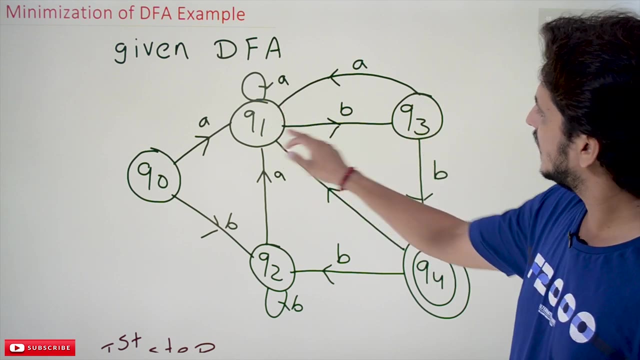 contains last characters are A, B, B. This A B B. that's the DFA. Let's take an example: A A, A, B, B, A, B B. Let's take this input string: A A, B, B, A B B. Yes, this string is accepted. We are moving to final state. 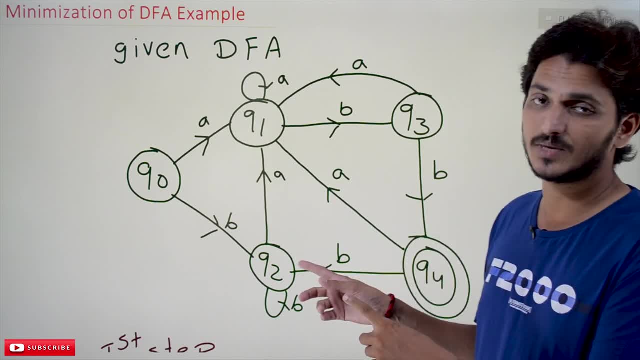 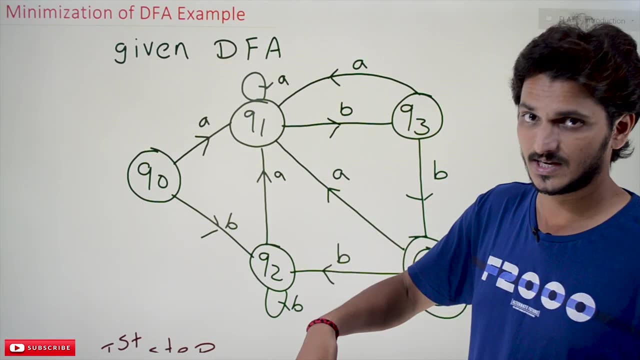 Minimize this DFA and we'll show that the same string will be accepted by the minimized logic also. You take any string, you check both the examples- this example and the minimized example- minimized output which we got after doing the procedure. Any string that is accepted by this DFA will be. 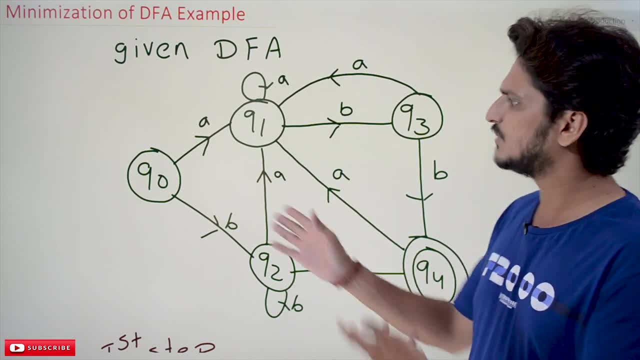 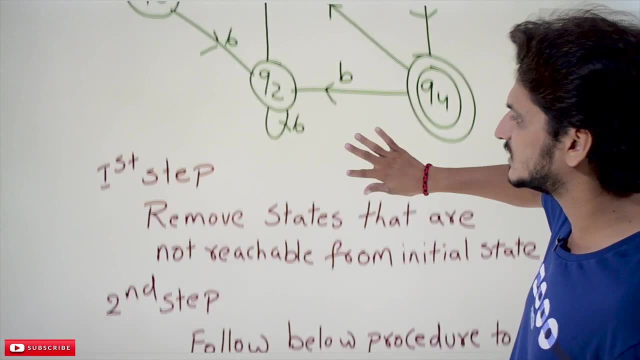 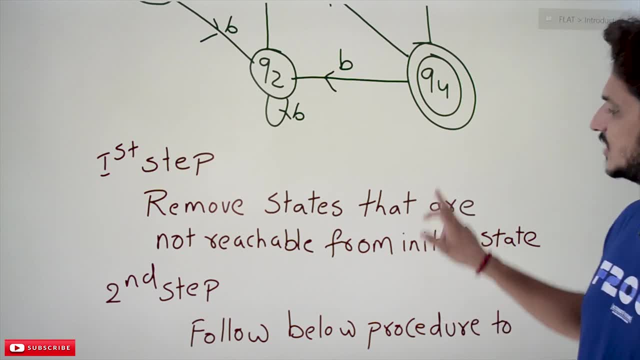 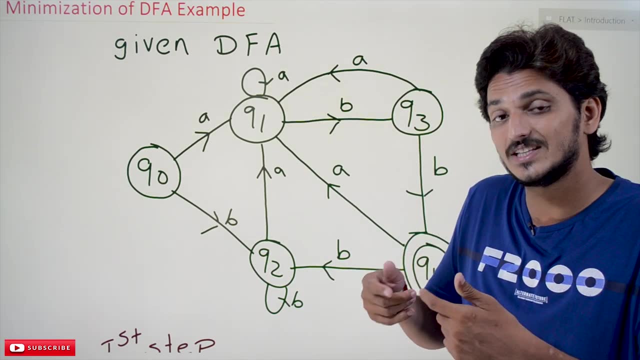 remove the string. We have to remove the string. We have to remove the string. You can also remove the string as well. You can remove the string if you are using aEST3 function that has to do with align 2 implementation. it can be. we can remove a OR that is selected. all that is welcomed from. 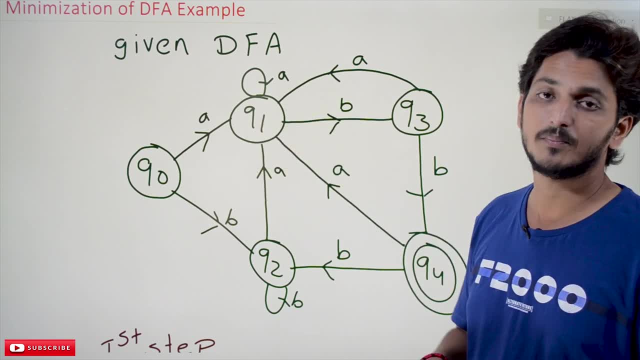 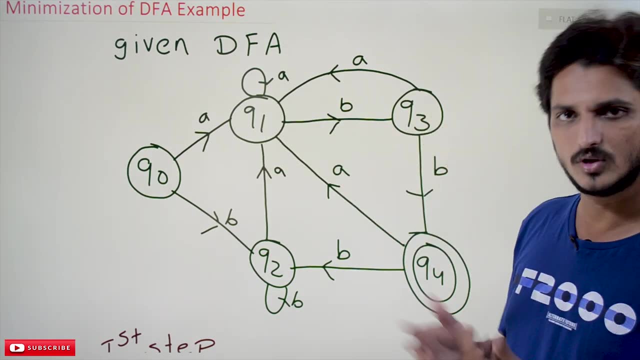 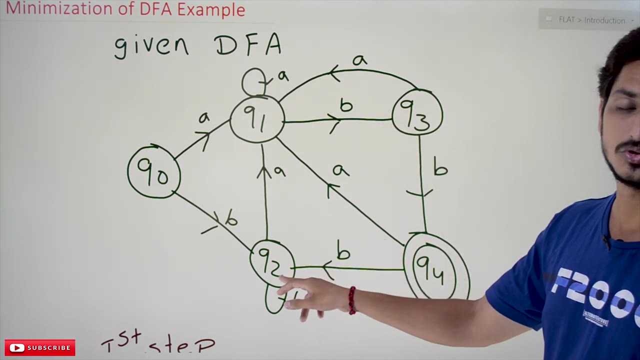 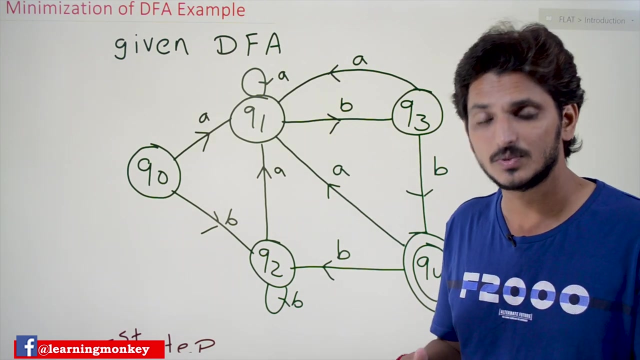 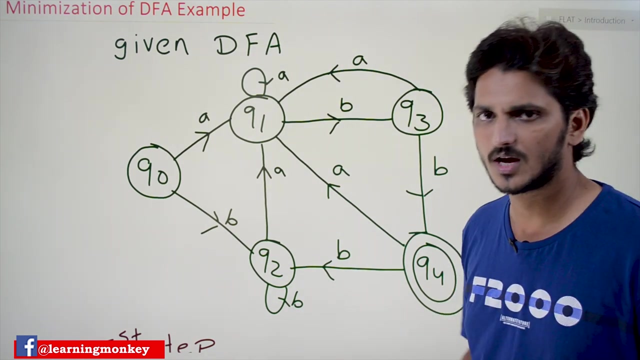 the table, which is that you can have a return in semiode. we can have a KEY of 7.. We can have a new chance when we are having. we will be able to solve it. So all the states are reachable. There are situations where some states are not reachable. Those examples will be discussed in our coming classes. next classes. Different variety of examples will be discussed in our coming classes. 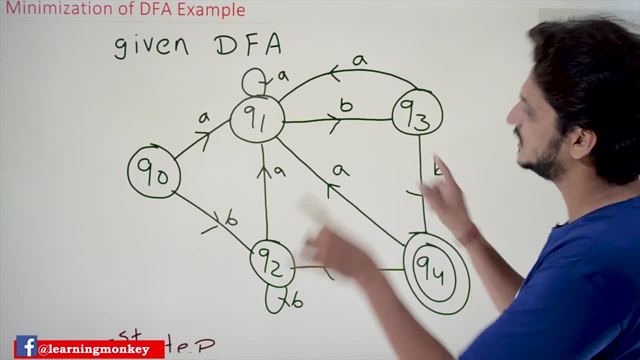 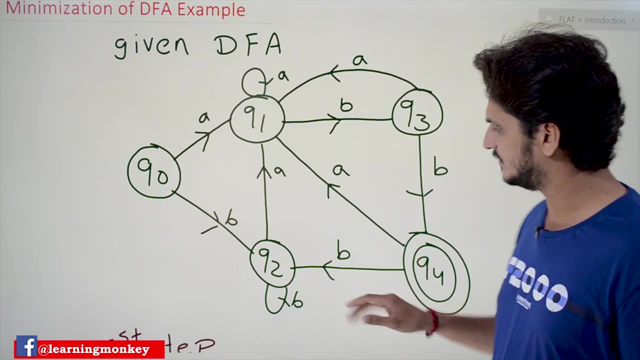 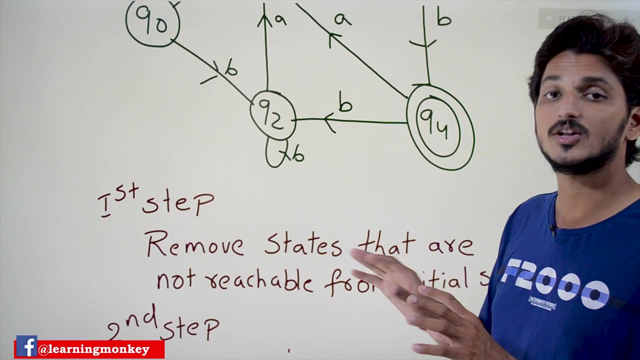 Now let's, for simplicity purpose, easy example has been chosen because this is the first class on minimization. To understand the process we have chosen the simple example Coming to the procedure: first step is eliminated because in our DFA we don't have any states that are not reachable from initial state. If there are states, we have to eliminate them. 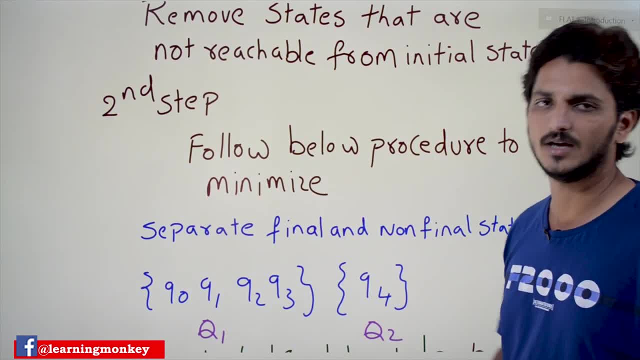 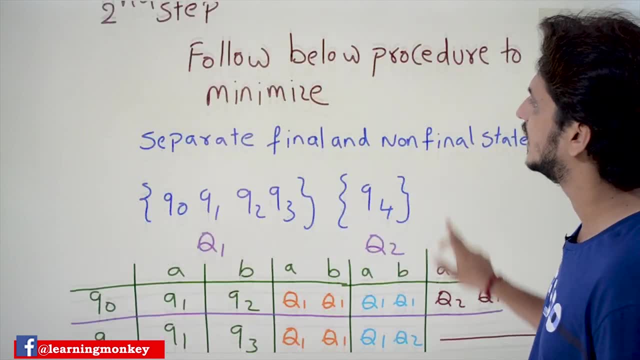 Coming to the second step, follow below procedure to minimize. So what's the procedure is? First, we have to separate final and non-final states In our DFA. what are the final states? Q4 is the final state and remaining are non-final states. 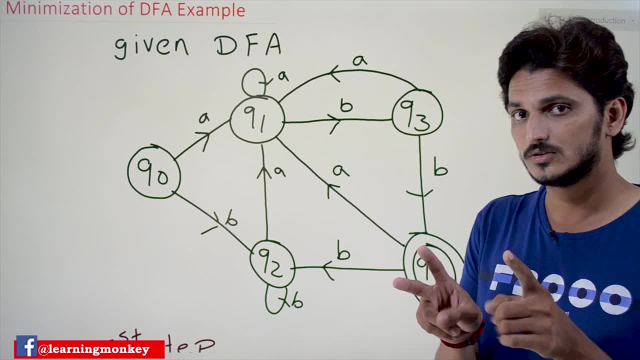 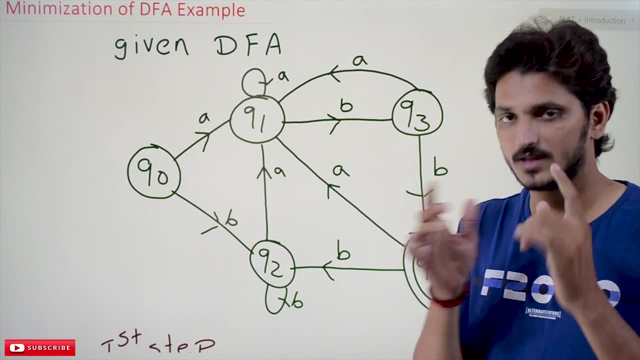 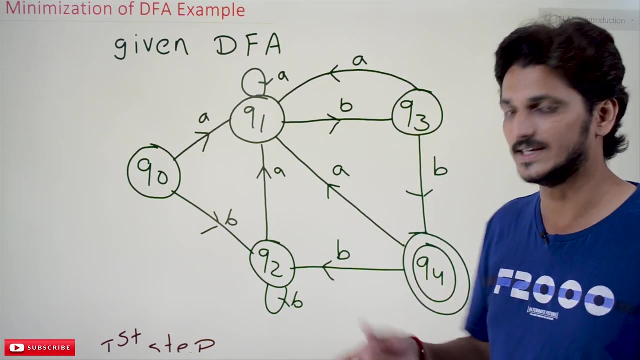 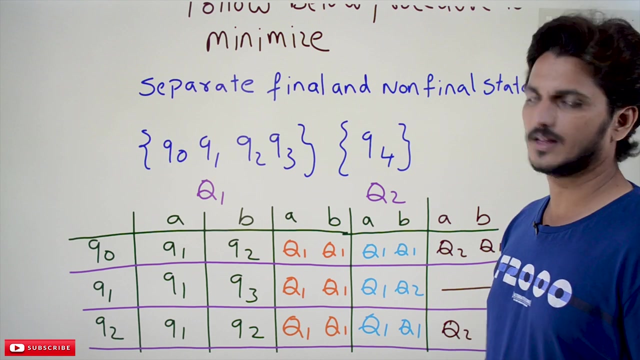 If you are having two final states, two final states comes to one set and remaining non-final states comes to other set. We are stressing on this point because this point will be helpful in our coming examples. So what are the final states and non-final states? Final state is Q4 and remaining non-final states are Q0,, Q1,, Q2, Q3.. 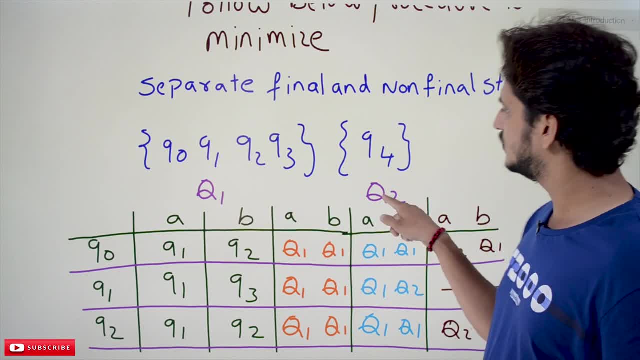 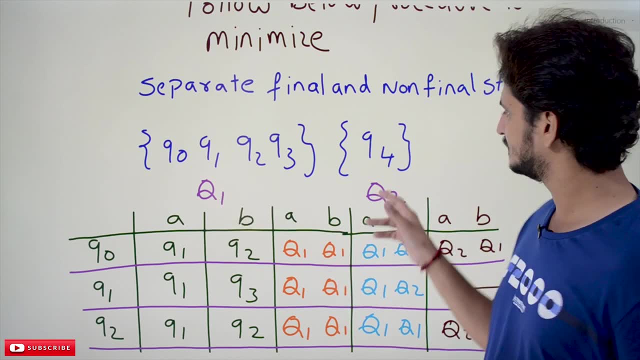 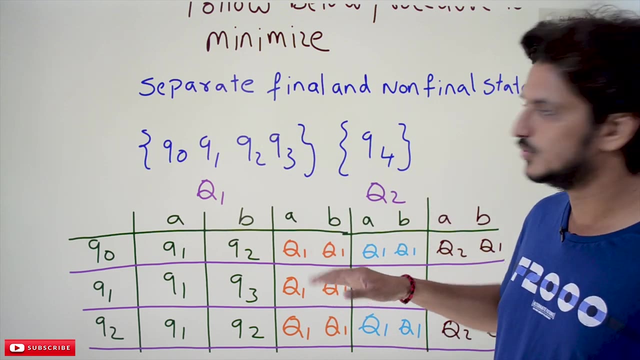 So we named it as capital state. This is set Q1, Q2.. This is set Q2, this is set Q1.. Whenever we say set means capital, Q is given the name, State means small, q is given the name. Now we have to follow a procedure to decompose these sets. 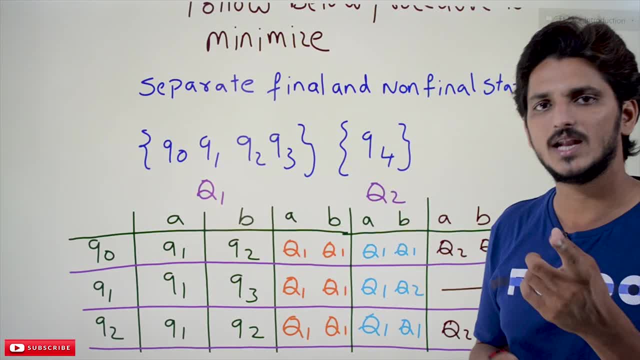 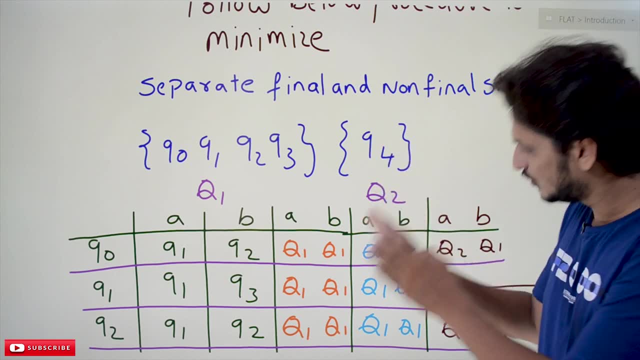 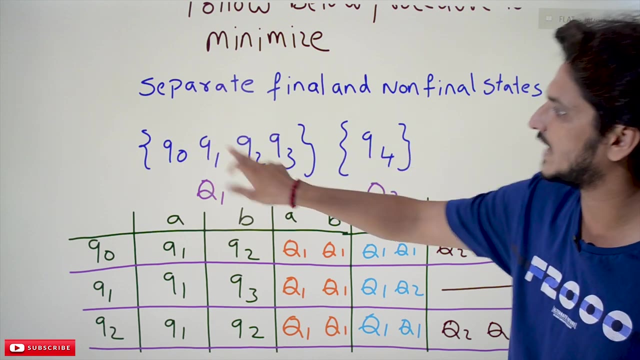 Can you decompose this set? In this set we are having only one element. We cannot decompose this set. So, whenever you are having single element, don't do decomposition, don't do the procedure. We cannot divide this set. We can divide only this set. This set Q1, because we are having multiple states. 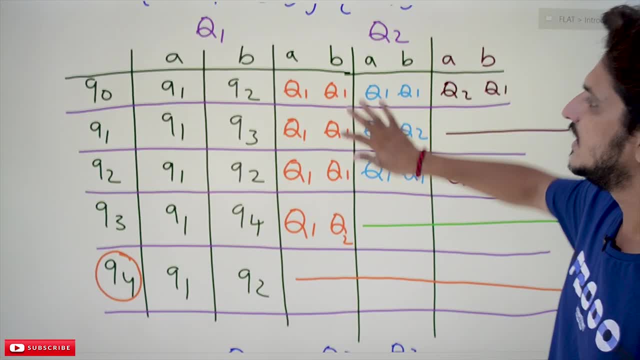 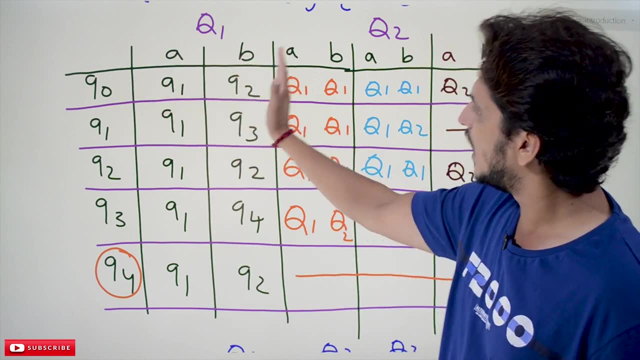 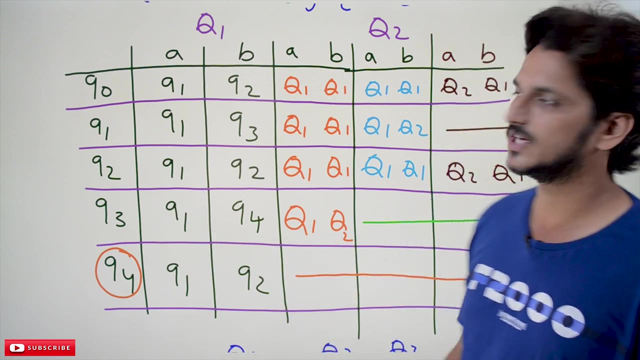 So how to decompose that, Let's try to understand. So these two lines is the DFA transition table Q0, A. we are moving to Q1, B, Q2. up to here. this is transition table From the transition table. this is the final state and this is the initial state. 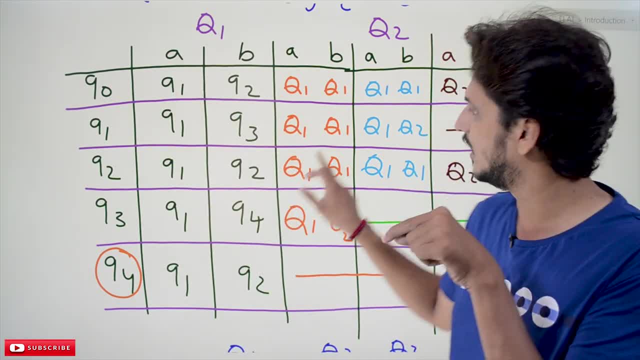 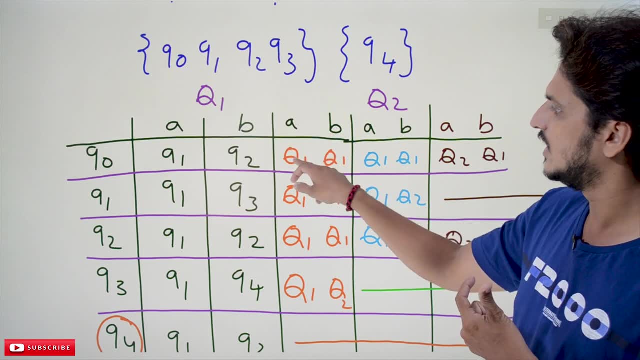 On Q0: if you apply A, we are moving to state Q1.. State Q1 belongs to which set Capital Q1.. That's what we have written here On applying A. we are moving to capital Q1. set Set Q1.. 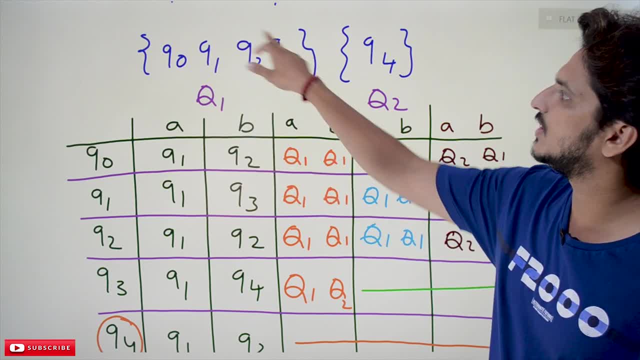 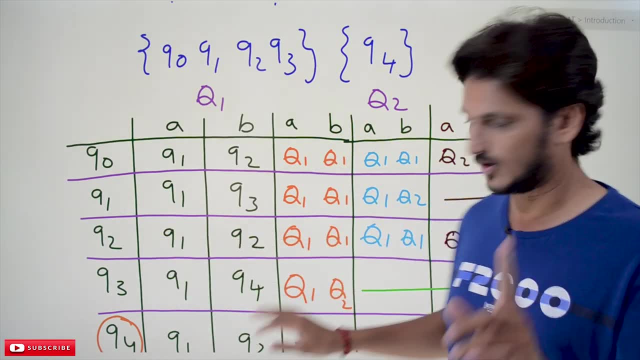 On applying B, we are moving to Q2 state. Q2 state belongs to which set Capital, Q1 set. That's why Q1, Q1 set The same way. repeat for all the states. All the states means here. on Q4, we should not repeat that. 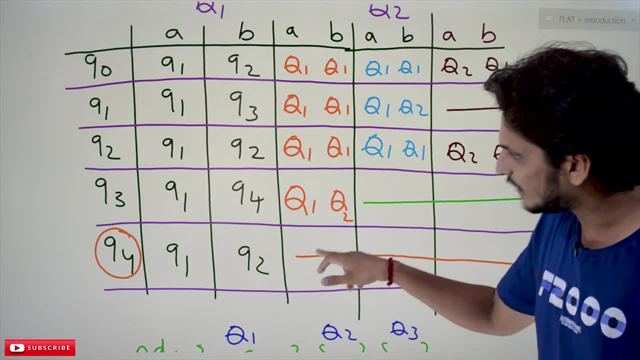 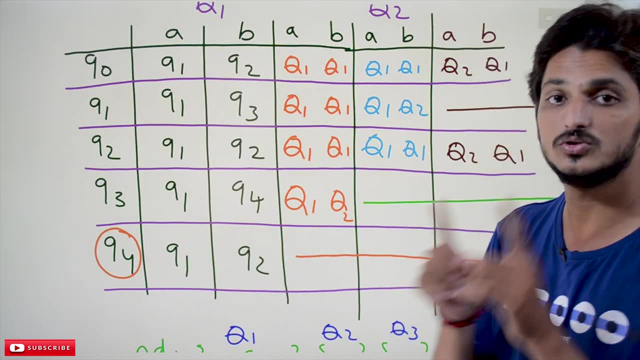 Remember that. it is very important. Most of them do mistakes. They will apply the logic here also on Q4 also, We should not apply that because this Q4 belongs to single element in the set Q2.. No need to decompose that. So that's why we have not written that. 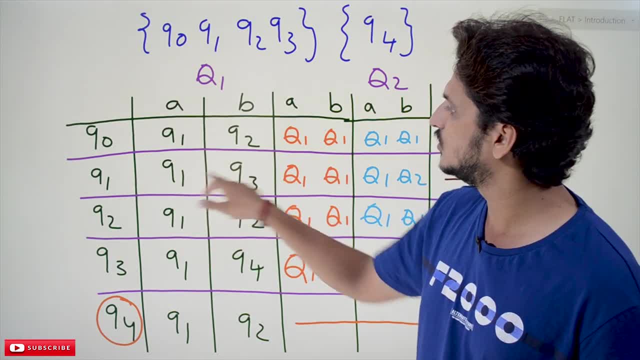 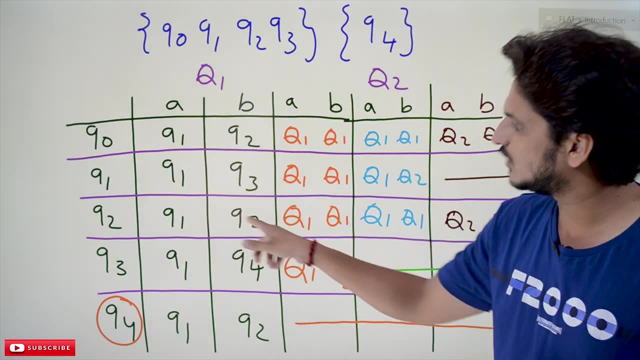 So the same way Q1. if you apply A, we are moving to Q1, Q3 state. Q1, Q3 belongs to Q1, Q1 set. Capital Q1, Capital Q1 set. Same way Q1, Q2 belongs to Q1, Q1 set. 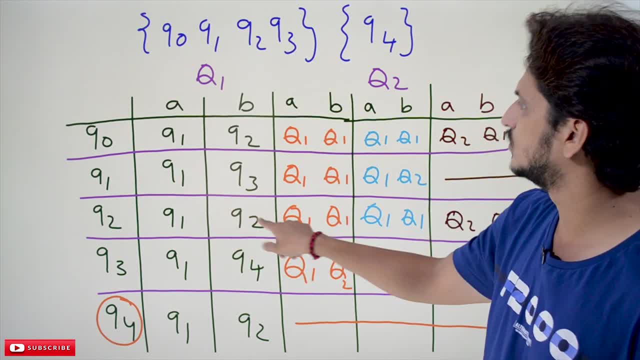 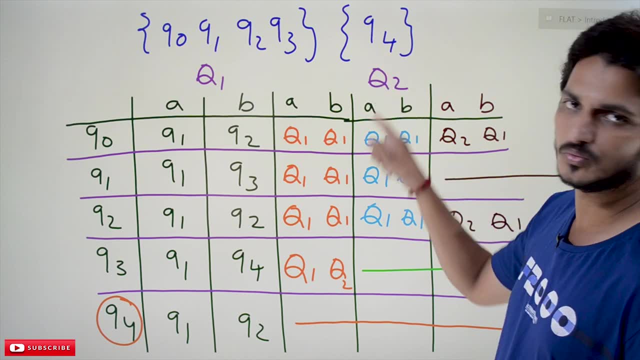 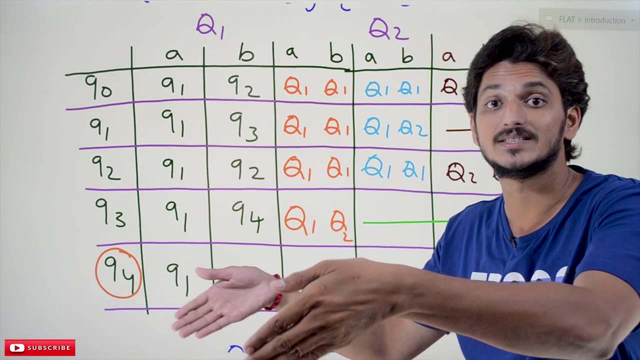 See Q1, Q1.. Q1, Q2 belongs to same set, But Q1, Q4 belongs to Q1 and Q2.. Q4 belongs to set Q2.. So out of these four, these three are going to the same sets. 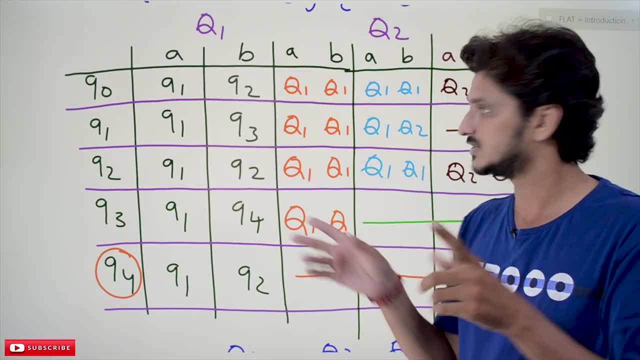 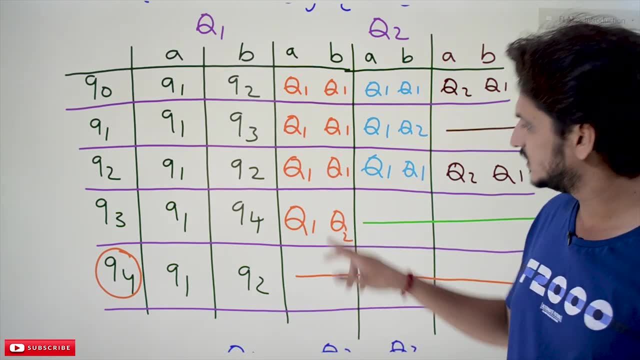 These three are going to the same sets. Remember this. Not states Same sets. Q1, Q1 is a set. Q1, Q1 is a set. Q1, Q2 is a. This is different, So separate it from the set. 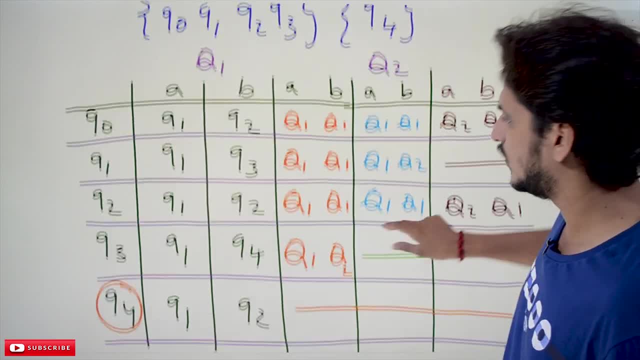 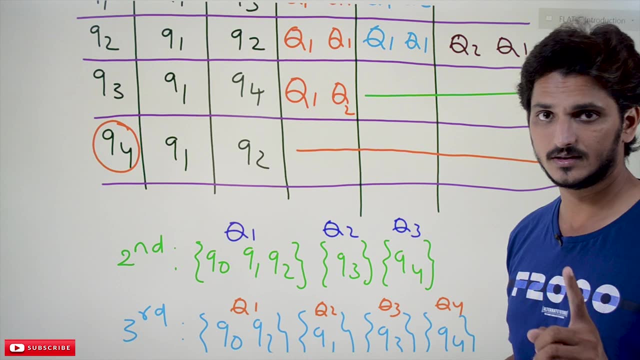 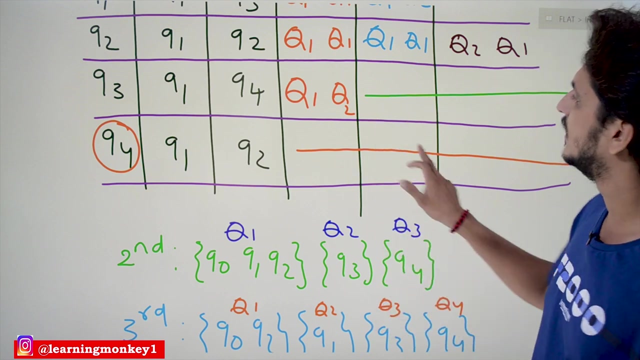 From this set, which one we have to separate. We have to separate the Q3 state. The new sets formed are Q0, Q1,. Q2 is one set, Q3 is another set, Q4 is another set. Q4 is already there in our beginning of the. 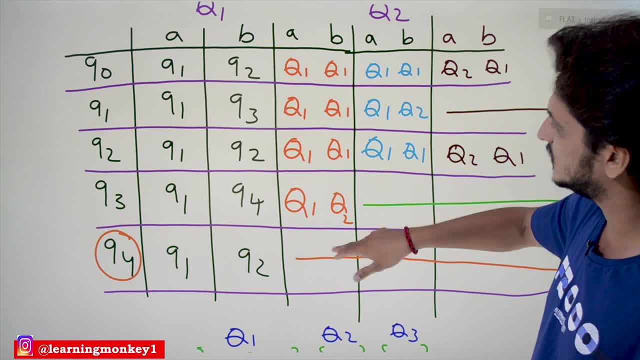 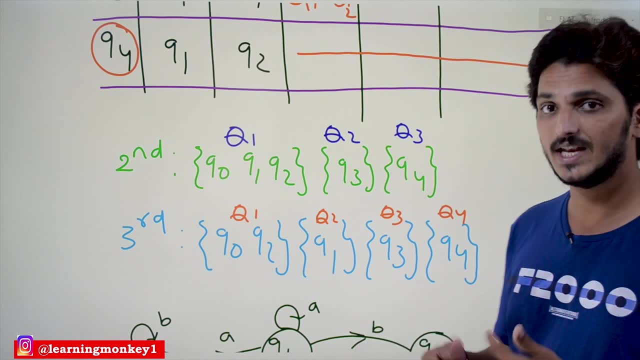 So first division is having Q4.. From this first procedure, first step. So what is the division we got? Q3 has been separated Again. name it, again name it. This belongs to set Q1.. This belongs to set Q2.. 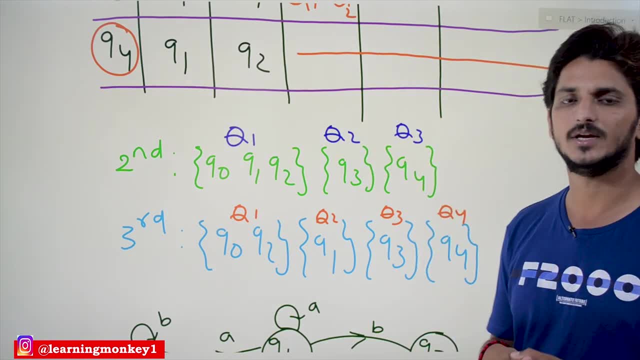 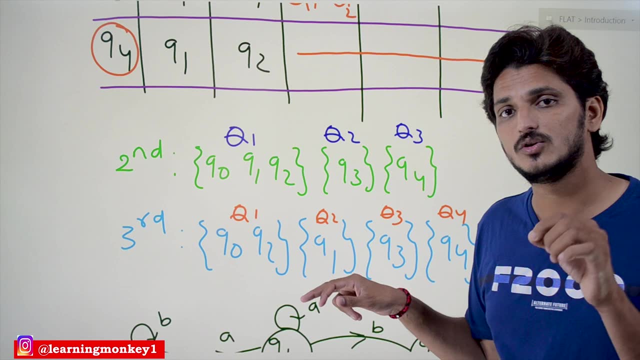 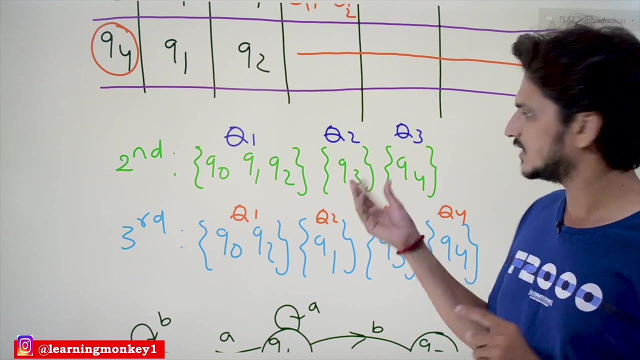 This belongs to set Q3. So we named it Again. repeat the process. Now we don't do it on Q3.. Why we are not going to do it on Q3 set, Not Q3 set, Q3 state? Because Q2 set is having single element. 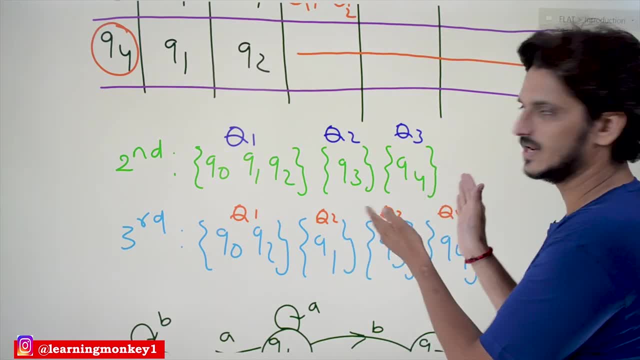 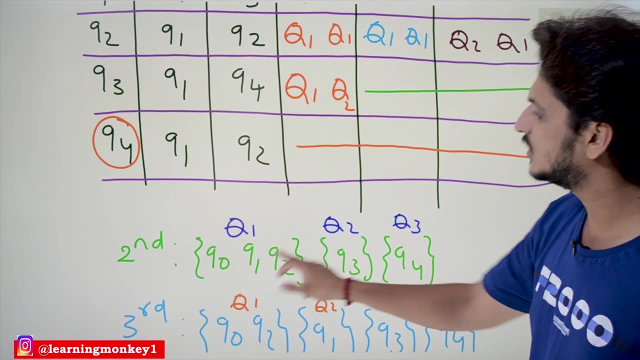 No need to divide. Q3 set is having single element, No need to divide. But we have to Decompose this Q1 set. That's why we will apply only on Q0, Q1 and Q2.. So that's why. 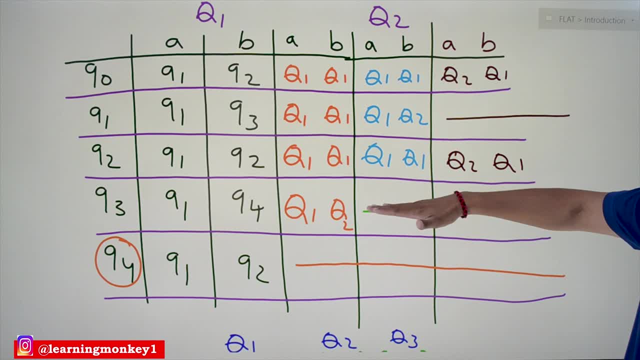 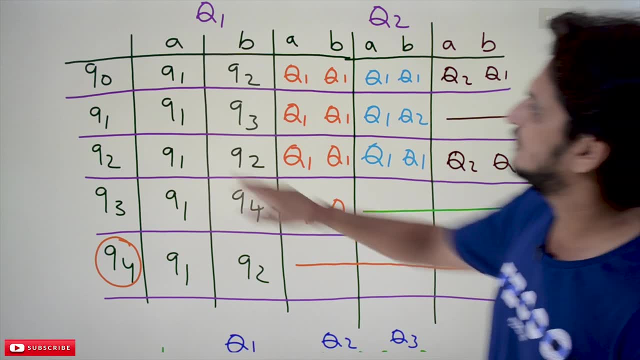 Here we have written the green line Because we are not supposed to do this In the second stage. Assume that this is stage 1.. Stage 2 and stage 3. The same way- Q0, if you take it as A. 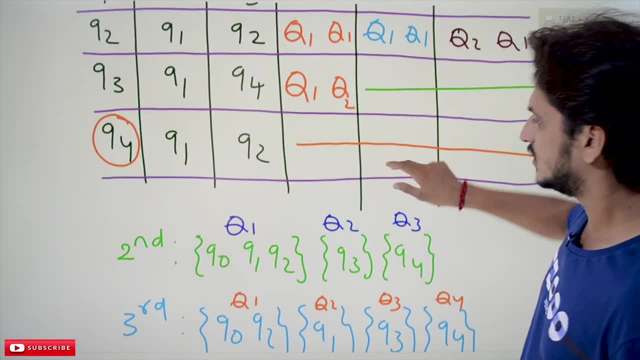 We are moving to Q1.. If you take it as B, We are moving to Q2.. So Q1, Q2 belongs to same Q1 set. That's what we have written. Q1, Q1. The same way. 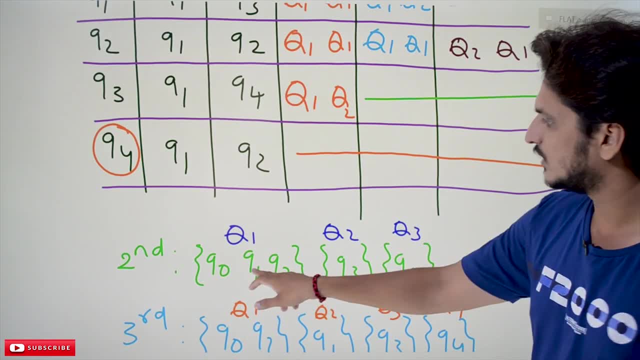 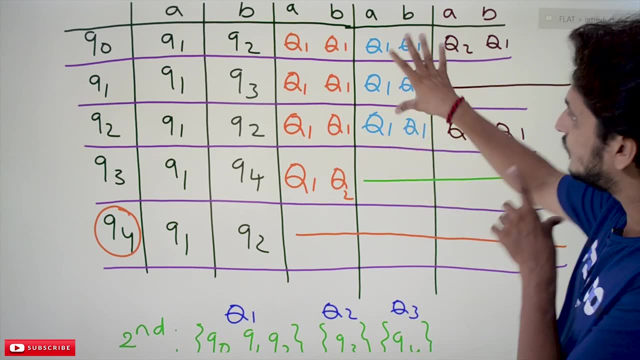 Q1, Q3 belongs to Q1 belongs to Q1 set. Q3 belongs to Q2 set. So that's why Q1, Q2.. Next one is Q1, Q1.. Out of these three, These two are same. 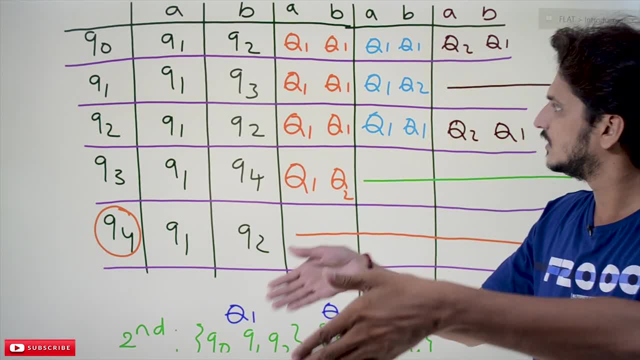 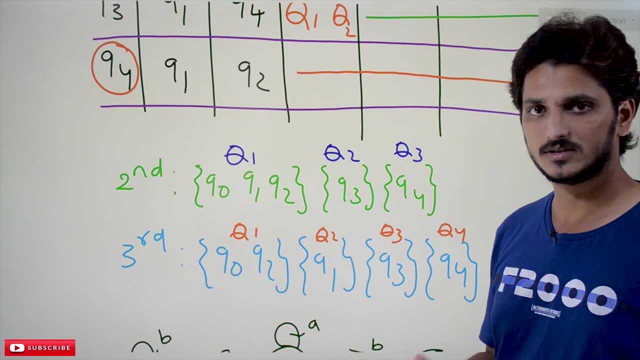 These two are moving to the same set. Okay, Q1, Q2 is separate. That's why Again split, Again split. What are the sets that are possible? Q0, Q2 is one set, Q1 is another set. 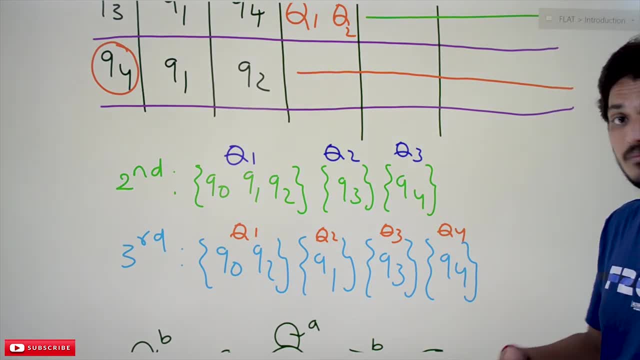 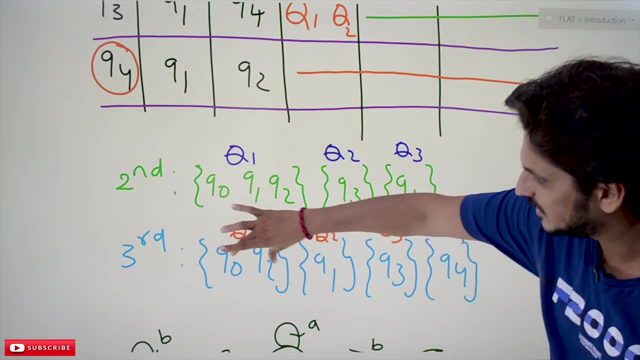 Q3 is another set, Q4 is another set. Again, name it. Again, name it. We named it as Q1, Q2, Q3 and Q4.. So on which states we have to apply the division? Only these two states. 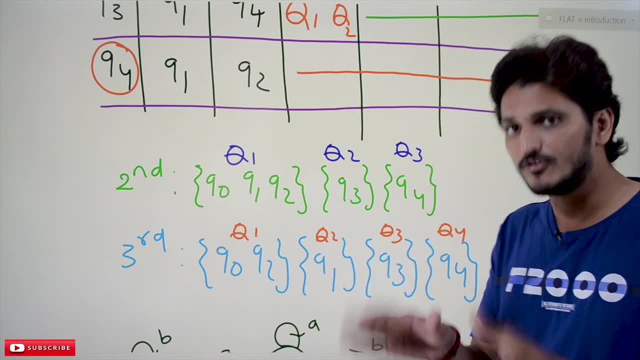 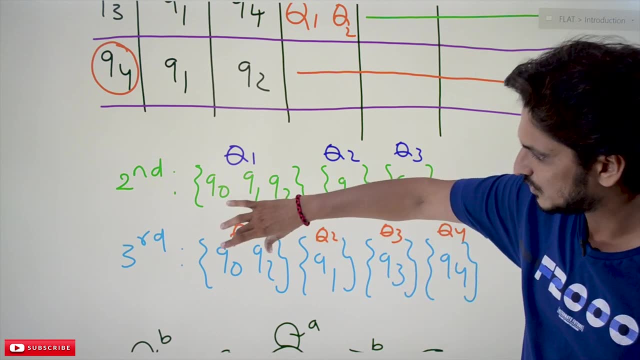 Here The point you have to remember First. suppose, First suppose In our process These two belongs to one set Means. We have to apply Q0, Q2.. And we have to check the division On Q1, Q3.. 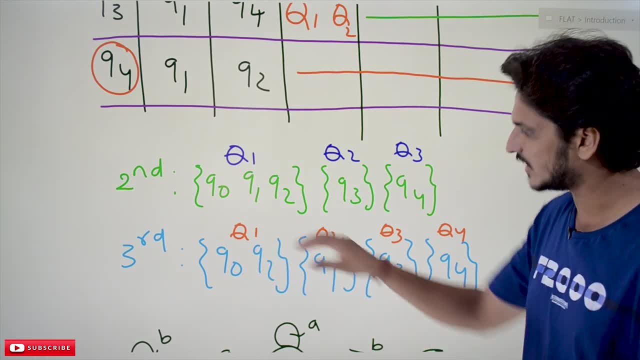 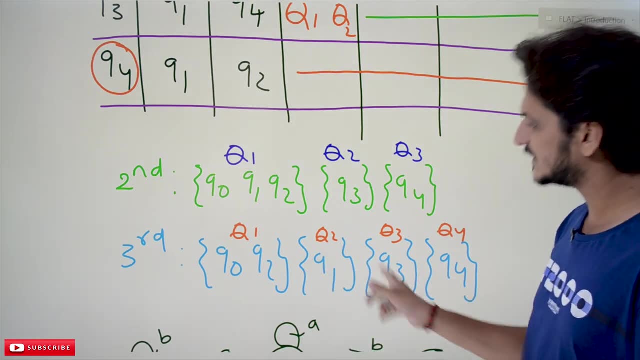 We have to check the division, But here we are having only one set That are having multiple states. So we apply on this Q0, Q2 state. So these examples also Having different possibilities also We will discuss in our coming examples. 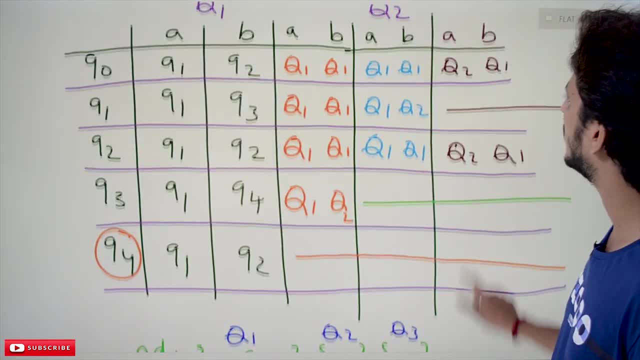 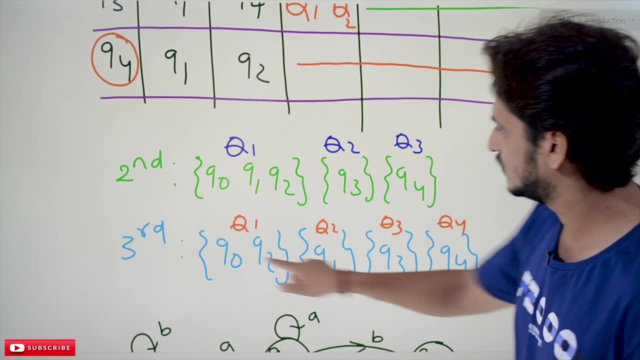 Again, repeat the process: Q0, Q2.. Apply on Q0, Q2.. Q0.. If you take Q1, set Q1, Q2.. So Q1 means set Q2.. Q2 means set Q1.. 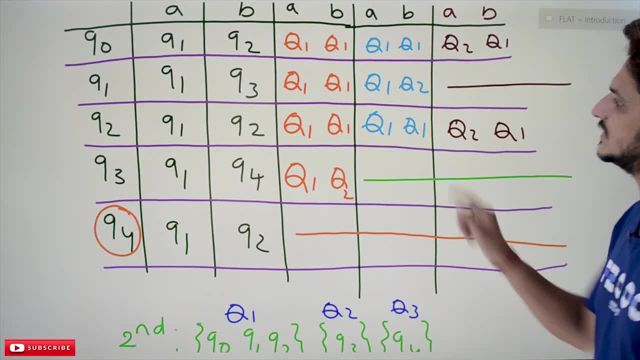 So Q2, Q1 set, Q2, Q1 set, The same way Q1, Q2.. Q2, Q1 set. It is not further divided. So we have to repeat this process Until our division is not possible. 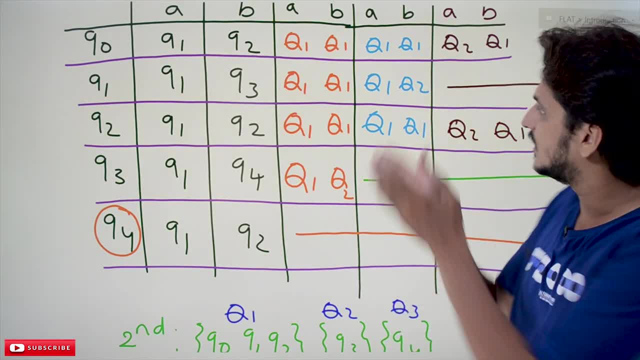 Here. we are not going to further divide our set. That's why we stop up to here. Now, what we have to do is The final sets are. These are the final sets Which we got. This is one set Means. What's the meaning of this set? 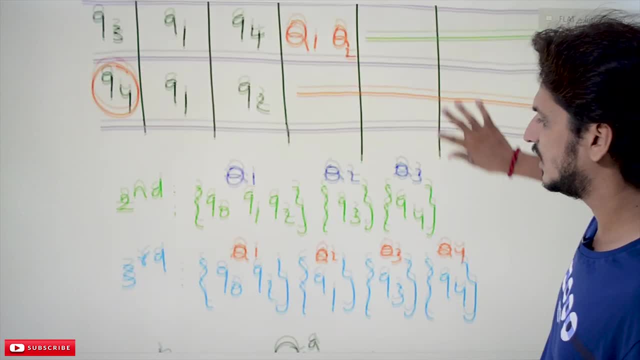 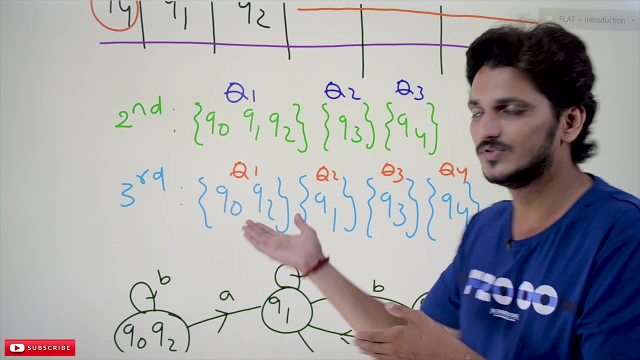 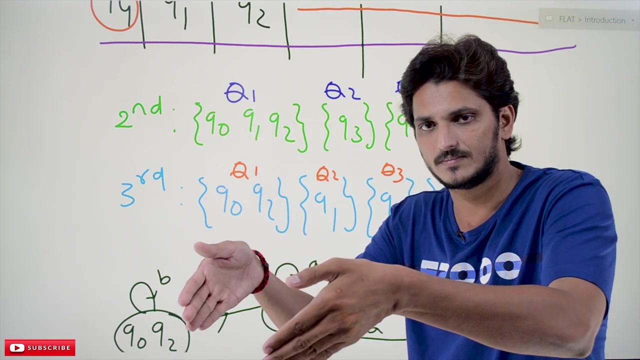 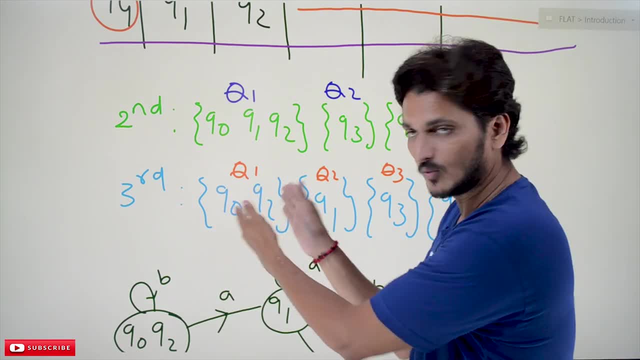 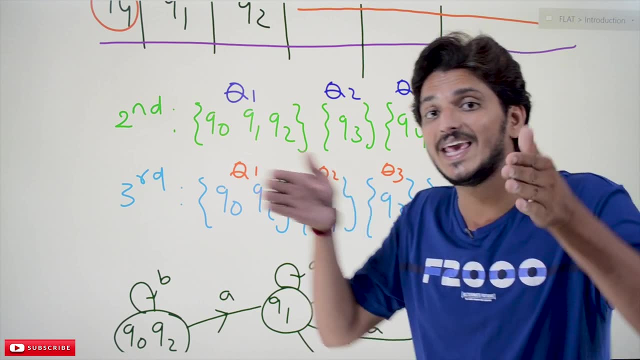 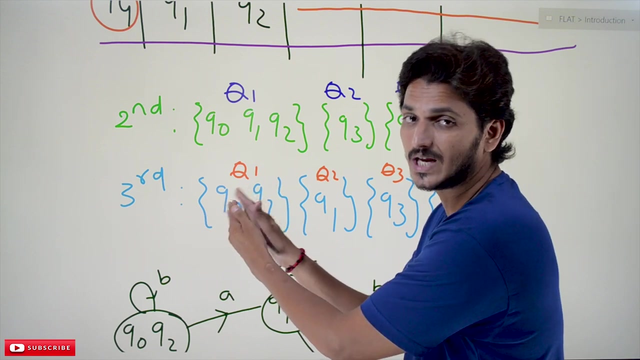 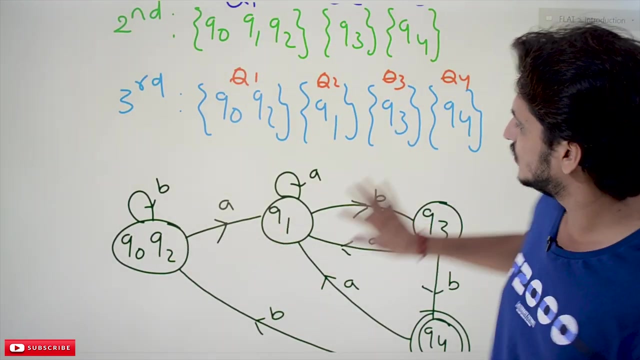 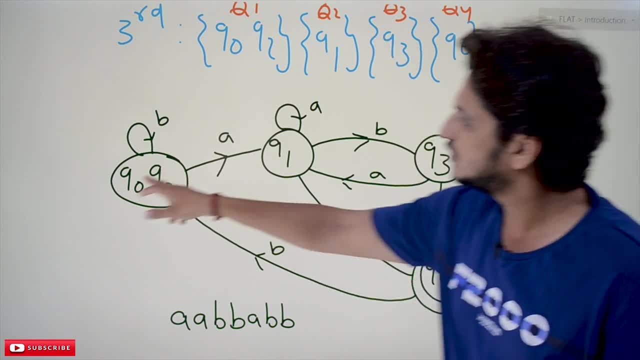 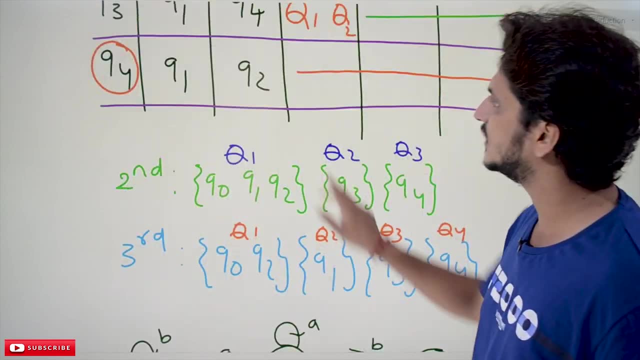 These transitions simply came from DFA table, So Q0, Q2 belongs to same set. We are combining these two states. So from the transition table: Q0, if you apply A, we are moving to Q1.. Q2, if you apply A, we are moving to Q1. 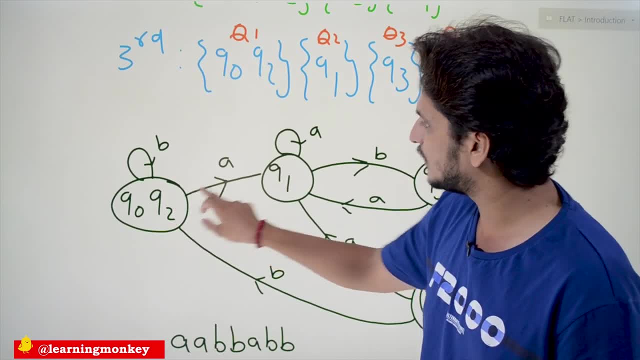 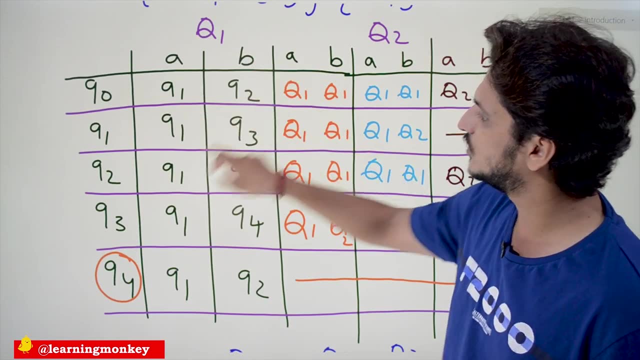 So that's why Q0, Q2 is one set. If you apply A, we are moving to Q1.. The same way from the transition table: Q0, if you apply B, we are moving to Q2.. Q2,: if you apply B, we are moving to Q2.. 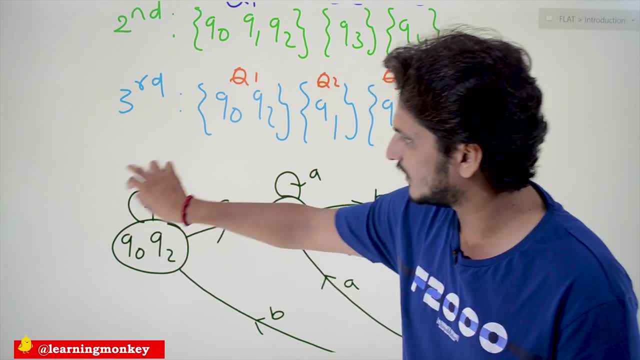 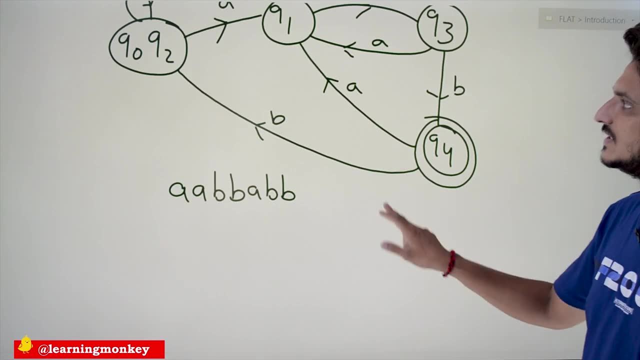 So Q0, Q2.. Q2 is in this set, So that's why we are moving to the same set. This is how we will combine the states. This is the minimized DFA. On this minimized DFA, if you apply the same input. 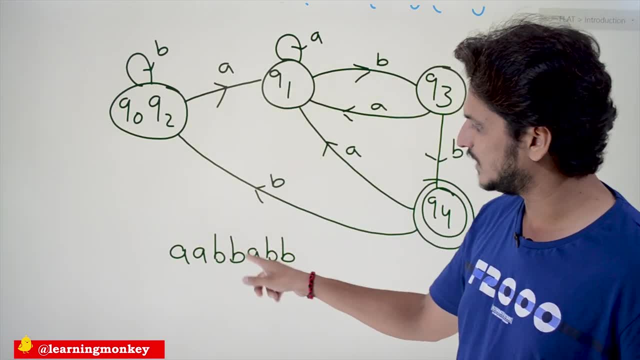 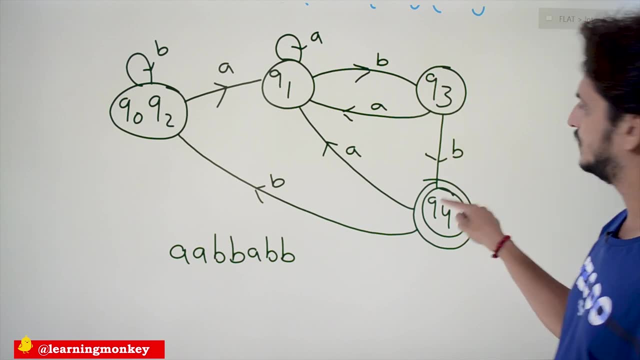 which we considered in our not minimized DFA- A A, B, B, A, B, B, A, A, B, B, A, B B. It is accepted. This is how we do the process for minimization. 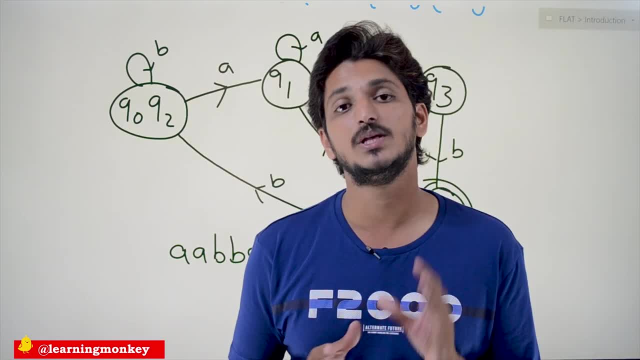 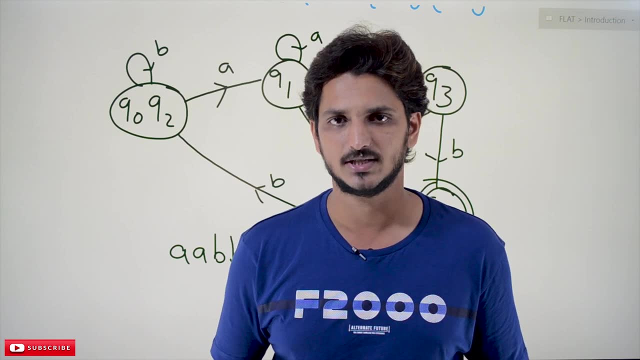 Hope you understand the concept. If you have any questions regarding the concept, please post your questions in the comment section below. Thanks for watching. If you haven't subscribed to our channel, please subscribe to our channel and press bell icon for the latest updates. 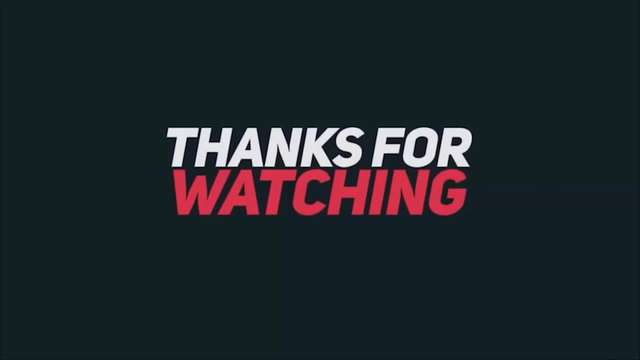 Thank you, Bye-bye.